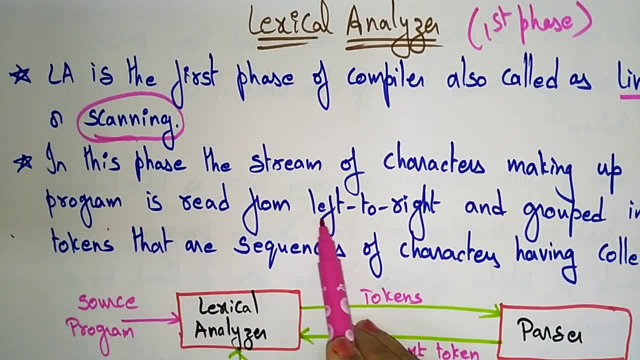 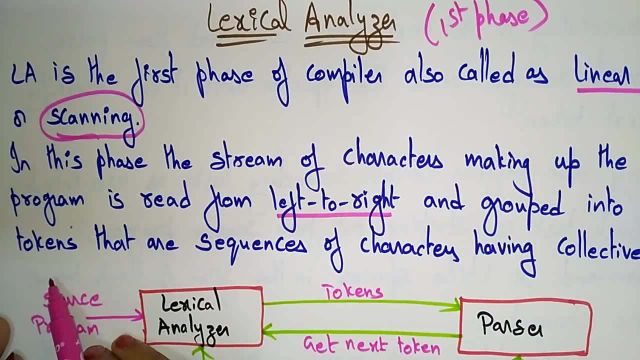 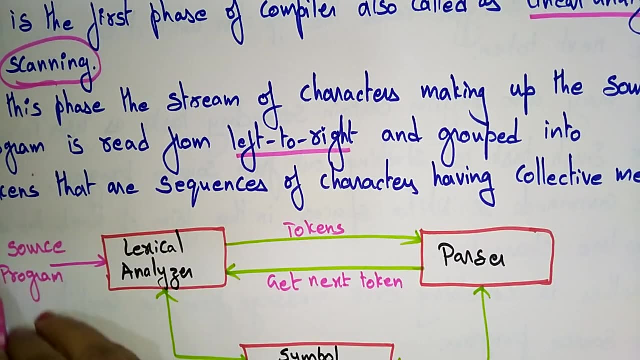 making up the source program is read from left to right. They are read from left to right and grouped into a tokens that are sequence of characters having collective meaning. Okay, So here, whatever the source program that is written in the high level language, that source. 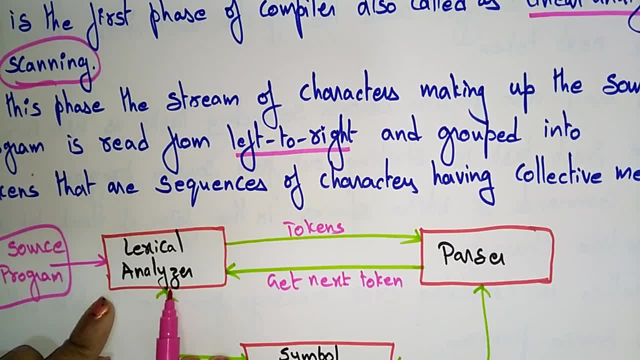 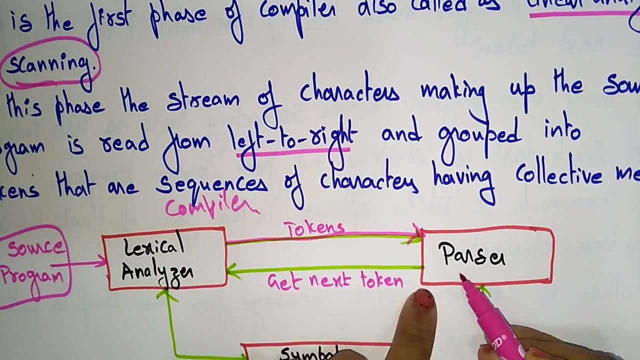 program is entered into the lexical analyzer in the compilation phase. So the lexical analyzer will convert the sequence of statements, characters, into tokens, Okay, And those tokens are enter into the parser. that is a syntax tree. So those tokens are represented in the syntax tree. So 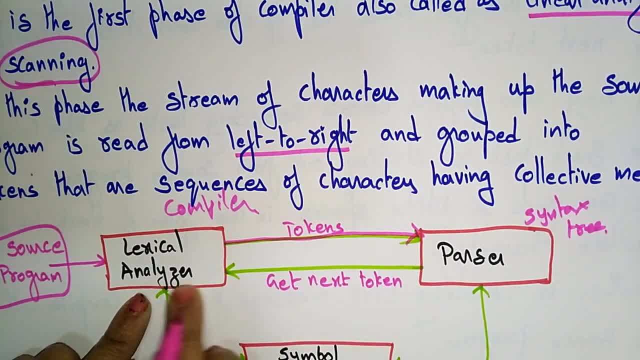 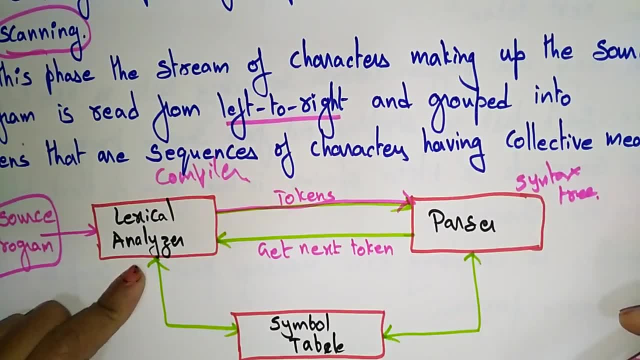 again, this parser is asking the lexical analyzer to send another token. So next, the lexical analyzer will send another token. like that, the tree will be represented. So here, the lexical analyzer as well as the parser. both are dependent on the symbol table. So what the symbol table is. 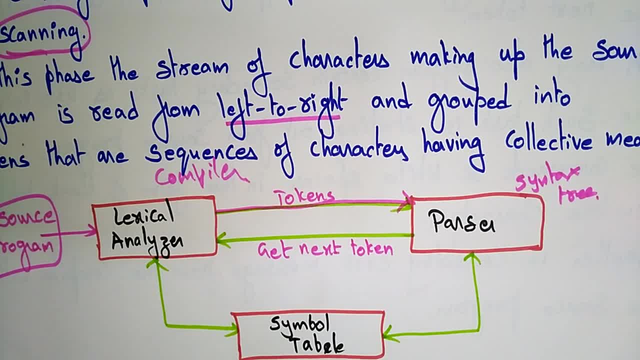 consisting of Symbol table contains all the identifiers names, along with their types, that are stored here. Okay, So that the symbol tables make it easier to the compiler or to the lexical analyzer phase or the parser phase to quickly search the identifiers records and they can easily. 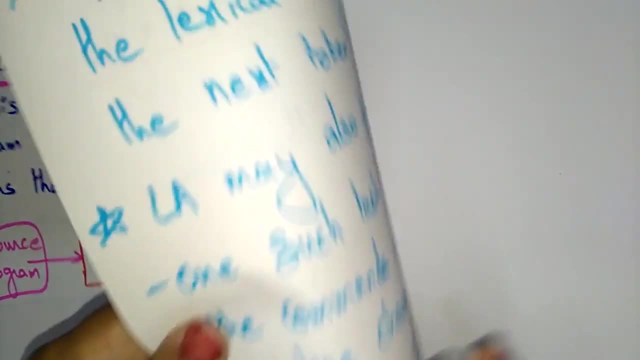 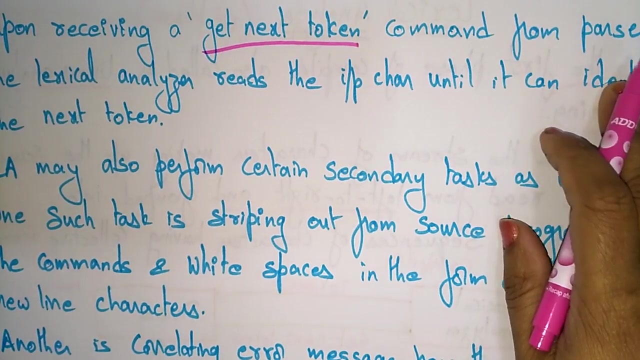 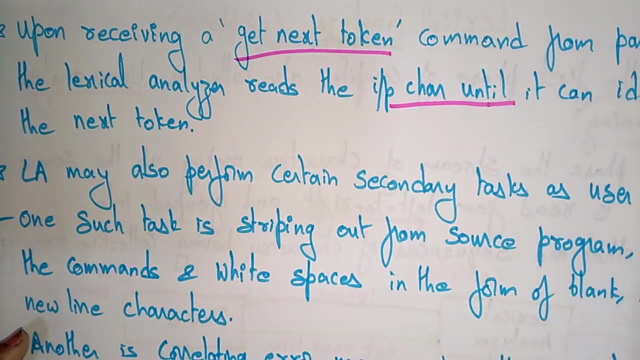 read: drive Okay And let's see upon receiving a get next token. So whatever the get next token, that is receiving command from parser, what the lexical analyzer will do. The lexical analyzer reads the input character until it can identify the next token. Until it can identify the next token, 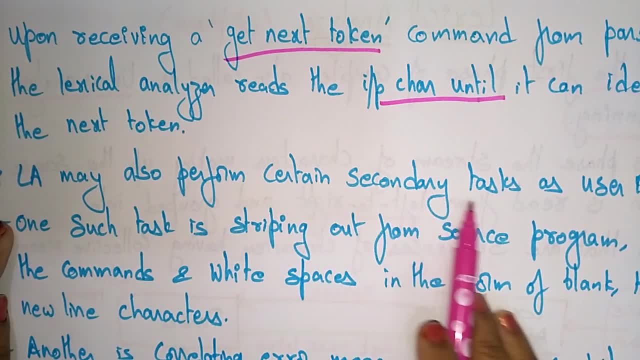 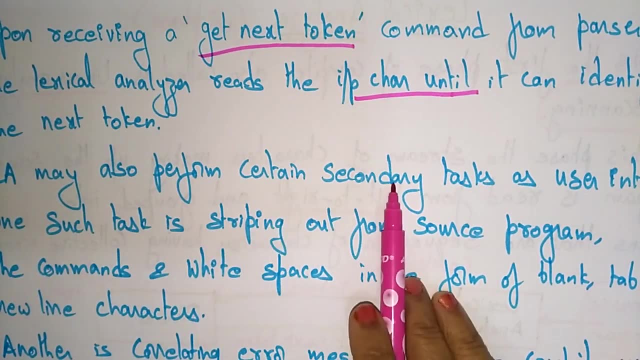 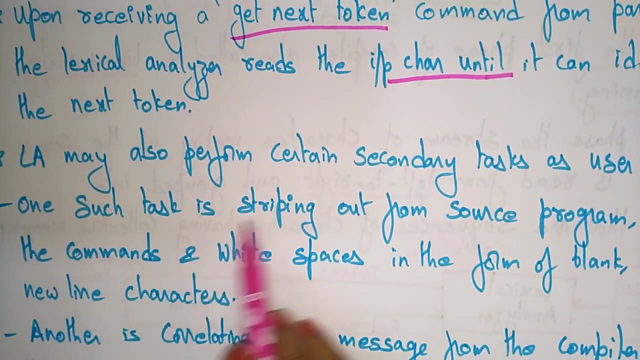 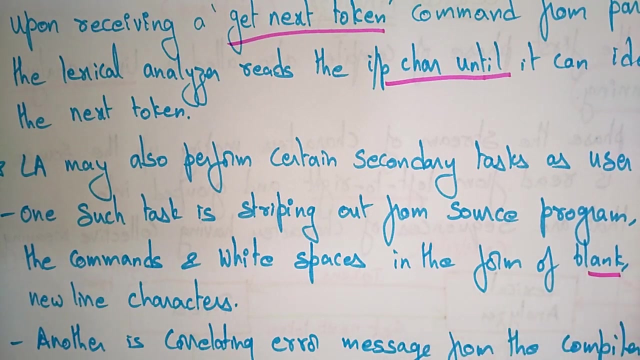 The lexical analyzer may also perform certain secondary task as user interface. So not only in. the lexical analyzer may also perform certain secondary task as user interface. The one such task is stripping out from source program the commands and the white spaces in the form of blank tab and